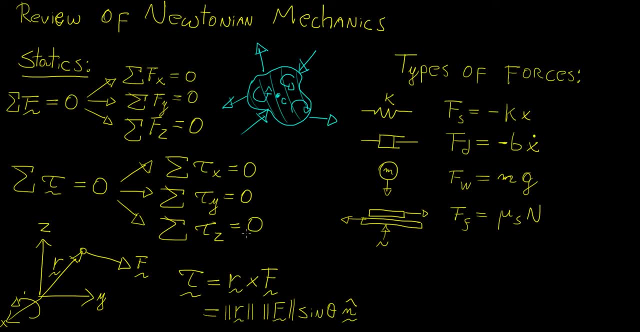 The components x, y and z and then adding them up. And of course, you know that the concept of torque in three dimensions is, if you have a position vector that gives you the position of particle with respect to the origin and then a force applied at that end, then the torque is simply the vector product or the cross product between the two vectors, which can also be represented in terms of the magnitudes, times sine theta and some normal vector to give you the direction that we need. 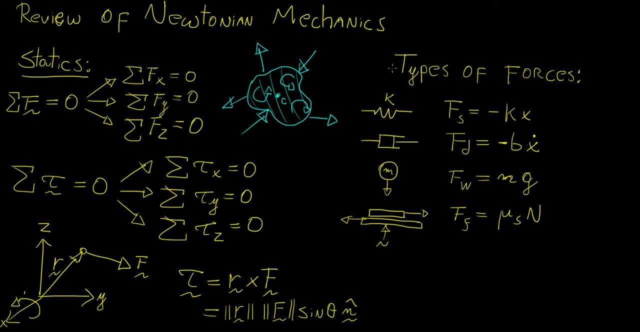 Now there are a few types of forces that we need to know of. So, basically, we have a spring force, which is essentially equal to the spring constant or the stiffness of the spring times, the displacement. Then we have a damping force. This one is more related to dynamics, but I have included it here because it usually goes hand-in-hand with the spring force. 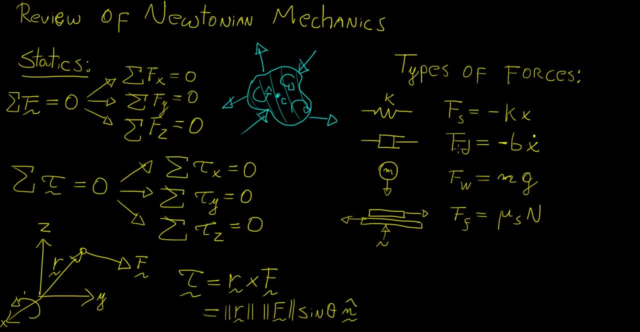 So you will see this in many, many different systems. So what is the damping force? Well, you have some damping constants, Which is just the equivalent of stiffness in terms of this force, and now you have the velocity. So basically, this is a damping force. The damping force absorbs energy. 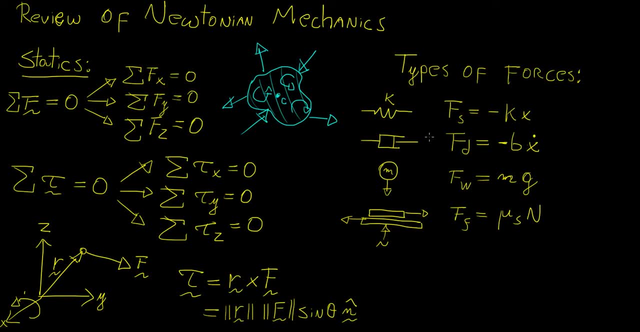 So you can imagine that if you have an object moving or oscillating back and forth, a damping force is actually absorbing energy the more that it moves, So at some point it just causes the object to come to a stop. Then we have the weight force, which we're all familiar with. 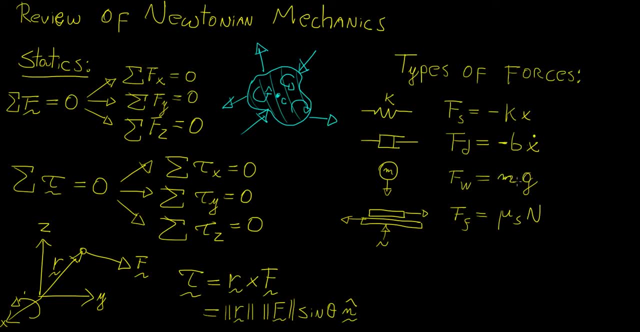 It is just the mass times the gravitational constant, So that's the weight And we have frictional forces. So for example, you can have the frictional force between two surfaces and you know that you can relate that to the normal force at one of the bodies times the coefficient of friction. 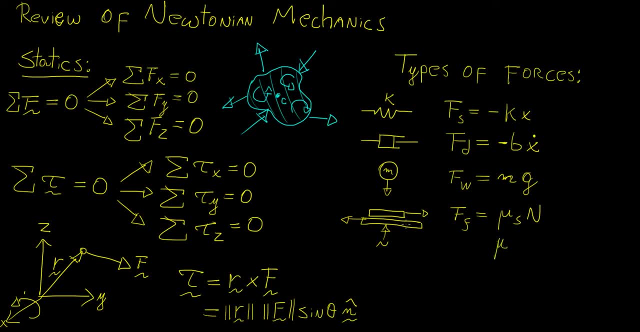 Of course you have coefficient of static friction in the case that they're both at rest initially, and coefficient of kinetic friction in the case that they're both moving with respect to each other. So there is a point of transition between the two. 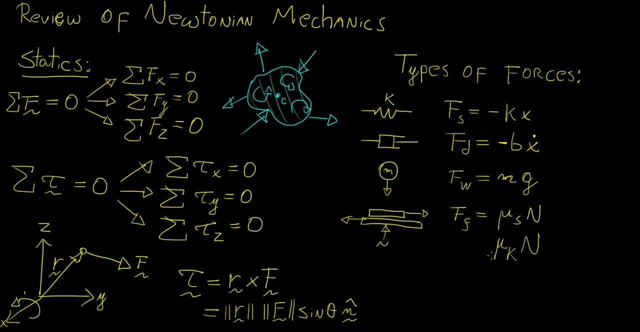 But we won't be dealing with this all the time, Because you will see that there are equivalent energy methods that can be used that kind of get rid of this kind of problem with transitioning from static to kinetic friction. Okay, so that's it for statics. 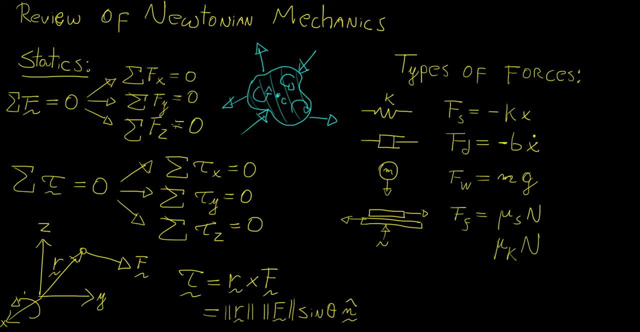 Those are the basic concepts. You have a bunch of equations, six equations that characterize the system in equilibrium. You have your three force equations, three torque equations. These are the different types of forces that you commonly encounter. You also have central forces. 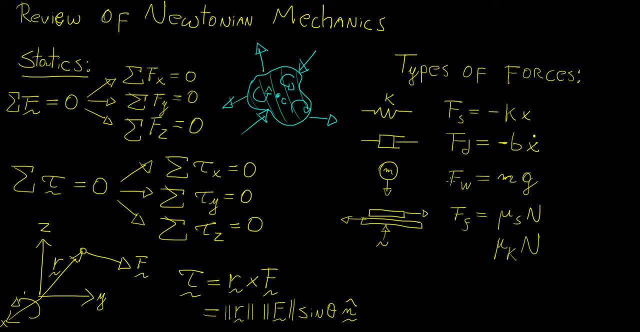 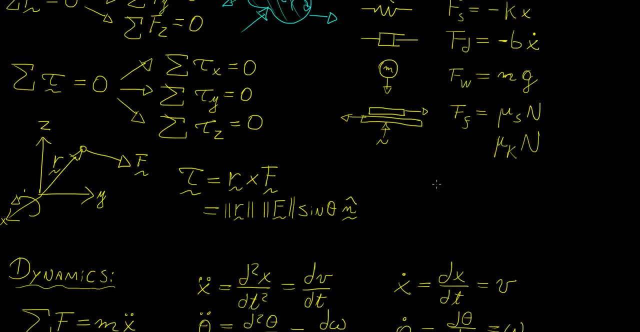 So you can have gravitational forces, electrostatic forces and so on, But we won't discuss those in too much detail. We're mainly focused with the mechanics of rigid bodies. Now in the dynamic section there are a whole lot of additional equations. 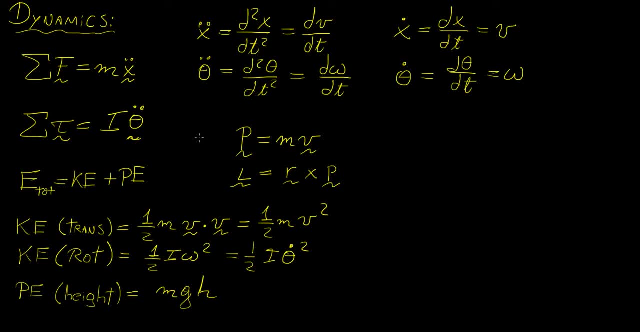 But here I have basically just written down the main ones that we're going to need. So in the case of a dynamical system, if you have a body that is actually moving through space, then in that case we take the sum of the forces and we make that instead of making it equal to zero. 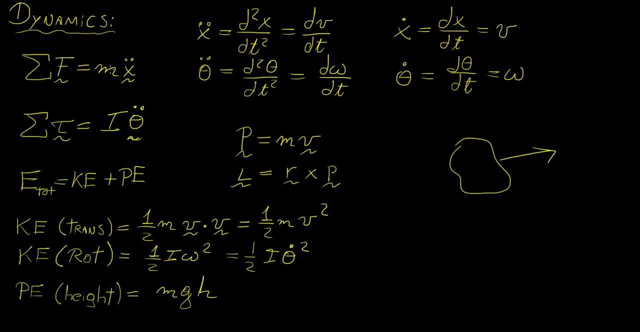 we make it equal to the inertial force, which is essentially the force that the body is experiencing about its center of mass. So you can imagine this force to be the total force acting on the body. So it will characterize the direction of the motion and basically how much acceleration is involved in terms of all those other external forces acting on it. 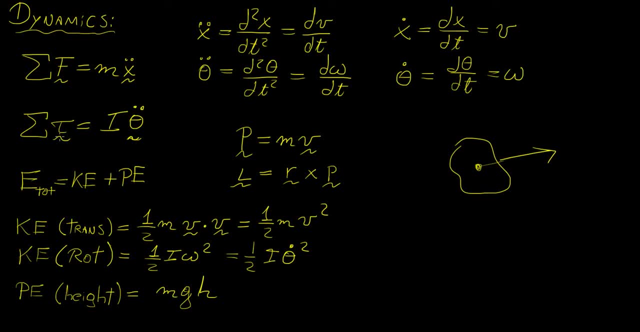 And we have an equation, Okay, And we have an equivalent expression for torque. So, because torque is just a rotational force, we have this quantity here called the moment of inertia, or mass moment of inertia, which is the rotational equivalent to mass. 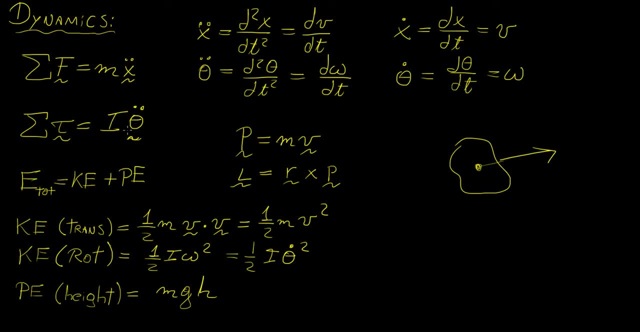 It is basically just resistance to rotational motion, And then we have this angular acceleration, So basically theta double dot. So I have included the definitions here. We know that this is the second derivative of angular displacement, which is just theta. And then those are the two main things that we do for force analysis. 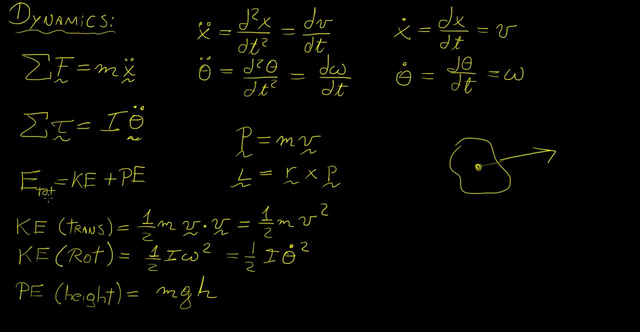 And then for energy, we can encounter the following formula: So we have: total energy of a system equals to kinetic energy plus potential energy. And then kinetic energy. there are many forms, but the main ones that we deal with are kinetic energy in translational motion. 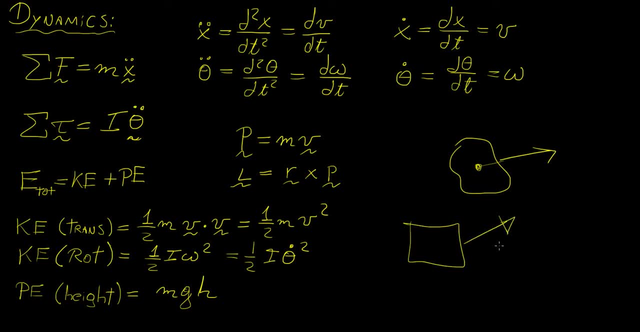 So basically you have a body and it is moving in a straight line across the all x, y and z axis And basically what you do is you take the velocity of the body, take the dot product with itself and that gives you this scalar quantity which is the kinetic energy. 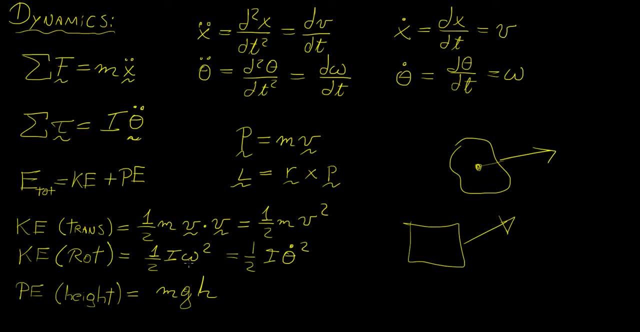 So this is something you are familiar with. Now, as you may imagine, there is always an analogy in terms of rotational motion. So basically, if you have a body that is rotating like this, then basically what will happen there is that the total kinetic energy of rotation is very similar to this formula, as you notice here. 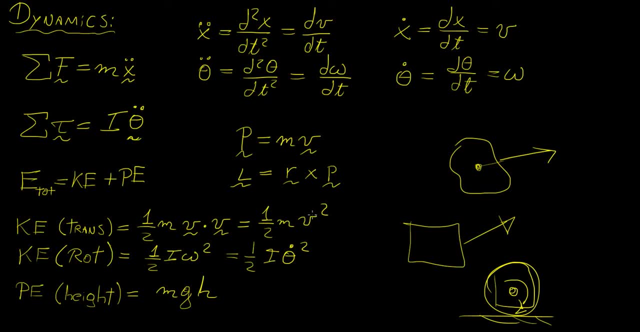 So instead of the mass we have the mass moment of inertia, And instead of the velocity we have the angular velocity, which is just the first derivative of angular displacement. So these two are going to come out quite a lot when we deal with like range and mechanics. 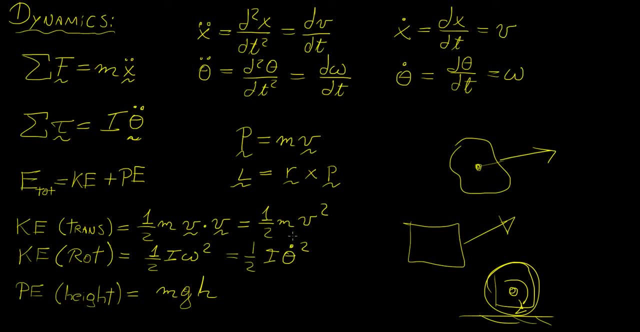 because these are the building blocks of the equations of motion, of the systems we will look at, And then you are going to have the potential energy. So, basically, the potential energy is defined for a whole bunch of different cases. So when you place an object at some height with respect to another body, 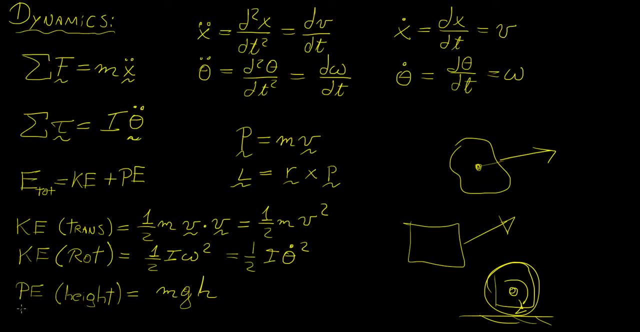 you have mg times the height, and that gives you a potential energy. There is another one that is quite common, which is the potential energy for a spring, And it is actually just the integral of the spring force with respect to the x, which actually gives you 1 over 2 kx squared. 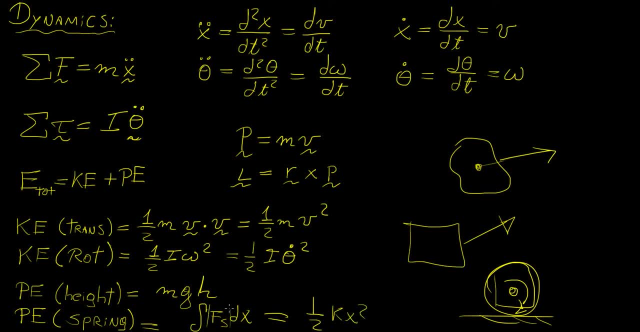 And the reason it is positive is because we know energy has to be positive. So we take the absolute value of that force and we get this expression. So those are the main things And, apart from energy, we know that we have momentum. 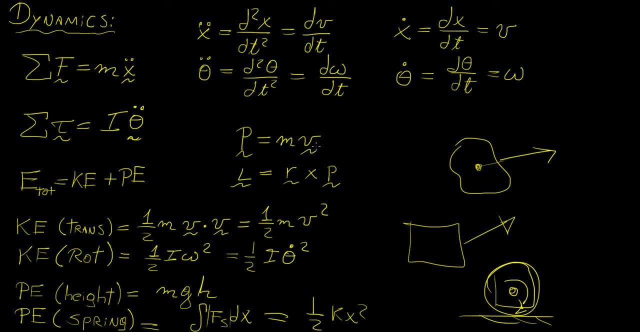 So momentum is essentially defined as mass times velocity. So basically it is just a measure of the effect of mass on the velocity of the body. And then the angular momentum is just the cross product of the position vector with respect to the momentum vector. 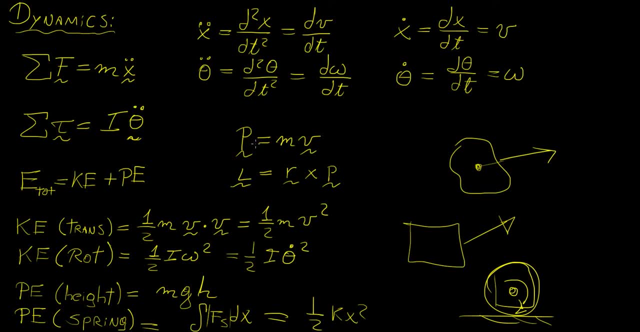 So you can imagine this is kind of like the torque analog of the linear momentum. We have these two quantities here, as you can see here. So those are the two main concepts that we have. There are, of course, a lot more other equations that I will pretty much just mention and explain as we go along. 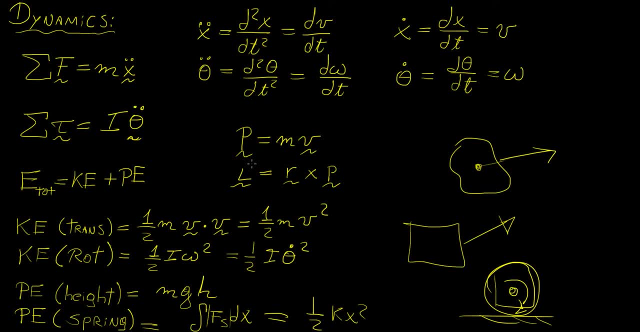 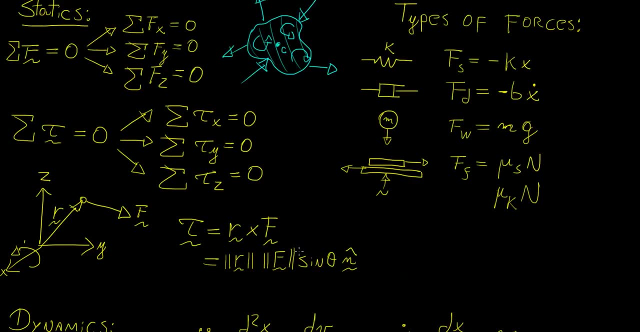 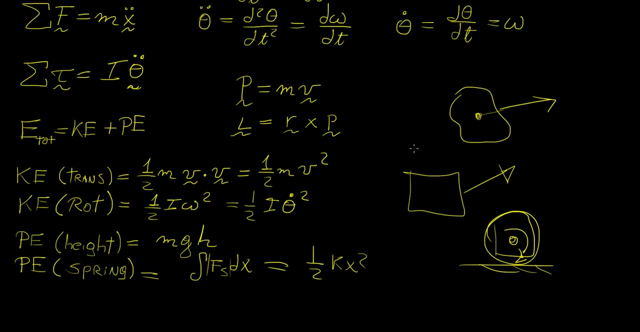 I won't get time to do everything in a single video like I have now, But I just want to make sure that you are familiar with these equations and these concepts, And once you understand what these things are all about, we can actually pretty much just get started on analyzing systems from Lagrangian and Hamilton. 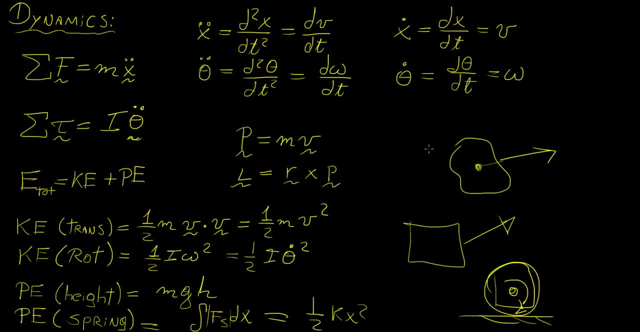 So in the next few videos I am going to introduce you to the mathematical formalism of classical mechanics, And after that we are actually going to analyze real systems using these new tools that we learned. 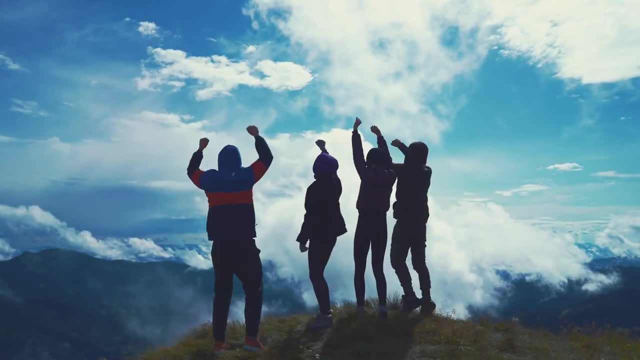 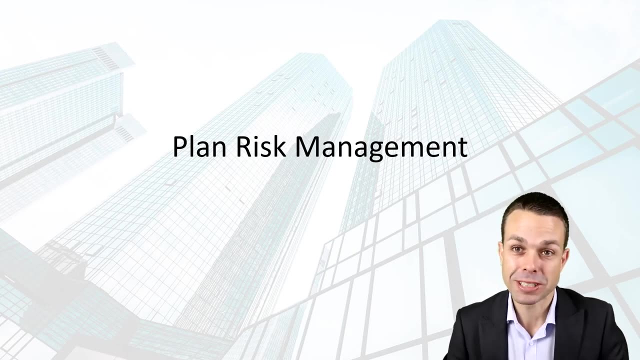 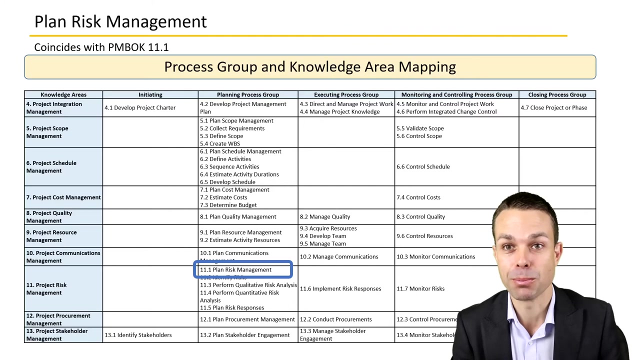 Hi everyone, welcome back to these processes from the project management body of knowledge. This one we're looking at is planning risk management. Now, where does planning risk management fall in the overall process group and the knowledge area mapping in the PMBOK guide? Well, as you can see, 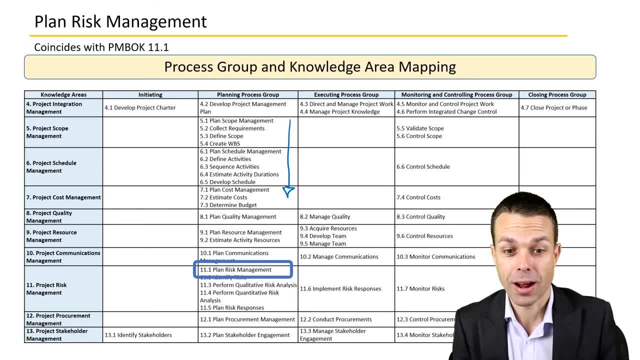 we're in our planning phase mostly- and you know there are other risk categories like implementing our risk responses and monitoring the risks as we're going along- but this is where we're actually planning the process of how we're going to manage the risk of our project and that's where we start. 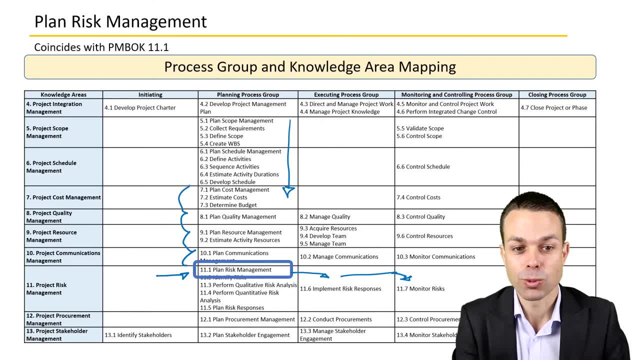 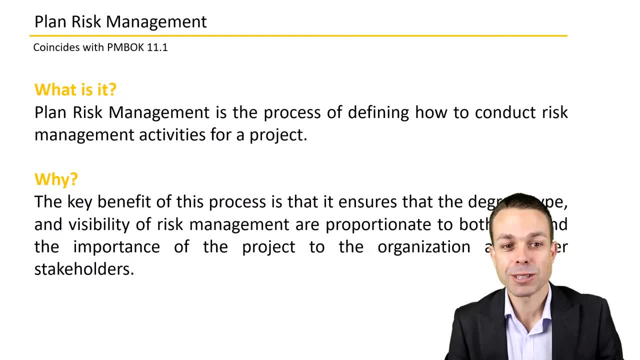 with our risk management plan and, of course, all these different plans will go up into our overall project management plan. as we know from previous chapters as well, Planning risk management is the process of defining how we're going to conduct our risk management activities for the project. 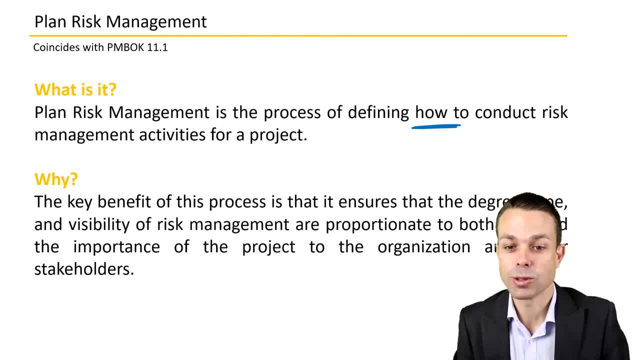 and the key benefit of this process is it ensures that the degree, the type and the visibility of all of the risk management activities that we're going to be doing in the project are going to be the same, as the risk management activities are proportionate to both the risks and importance of. 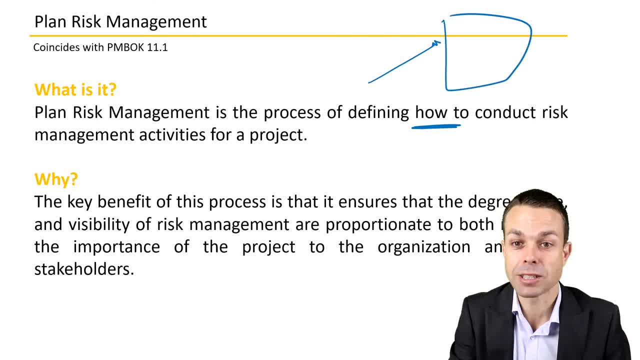 the project. So if it's a large project- maybe it's a big, big project- then maybe we need a large risk function within our project. We need a lot of- you know, more people, maybe a particular a group of people, to be focusing solely on the risk. or, if it's a small project, maybe all of these risk activities.